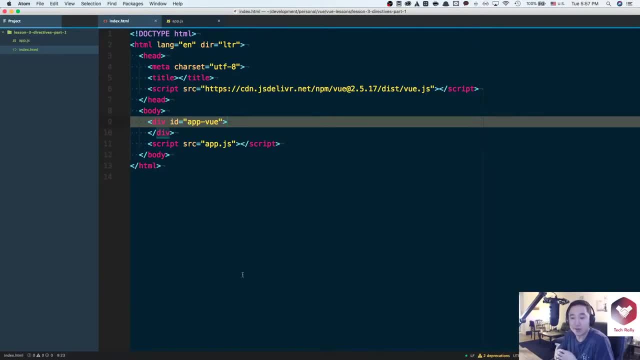 I've already created the same folder structure as lesson two, so I would highly recommend doing the same template and JavaScript file for this lesson. Like the lesson before, I'm going to be using the root element called app Vue. Inside of the app Vue div container is where all my 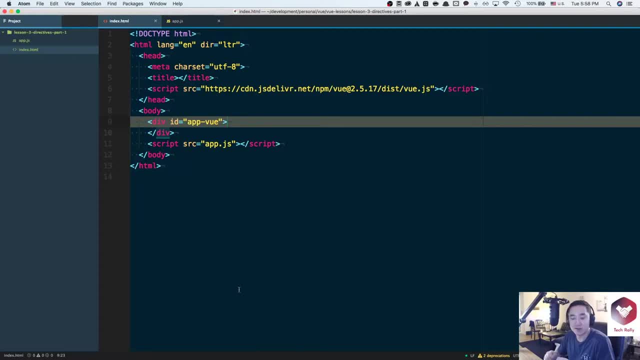 directive logic will be. So let's start on the directive app Vif. For display purposes I'll use a header tag to kind of separate how each directive logic works. So in the beginning I'll just create an empty container. So here I've got java4, Vif and then we'll create another separate container called H4, Vshow and 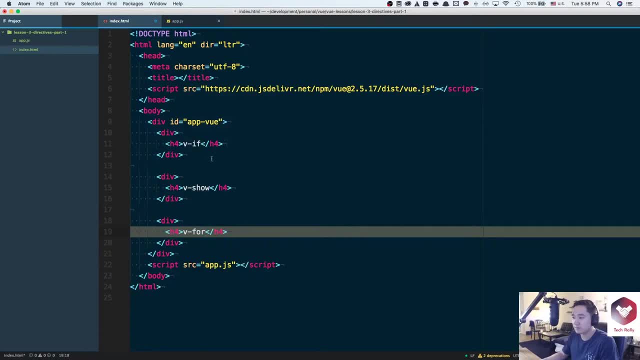 then separate container here called V4. And then actually in here we'll just say Velse as well, And this is just plain HTML. Now let's go back to our JavaScript code, and it's just like an empty file. but we like the lesson. 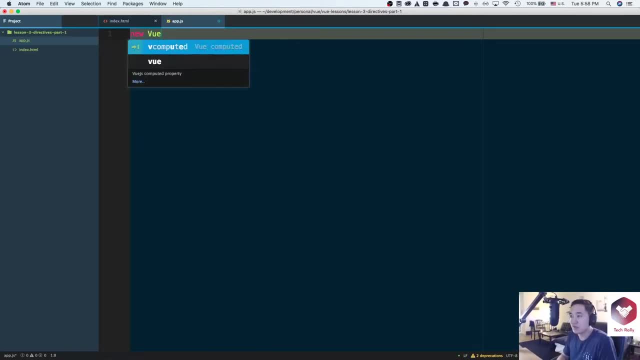 before we need to create a Vue instance. We're going to do that- a new view- And then we create an L key and point it to the ID of the root element, which is app view, And then we'll add more data to our instance And here we'll return some kind of data set. 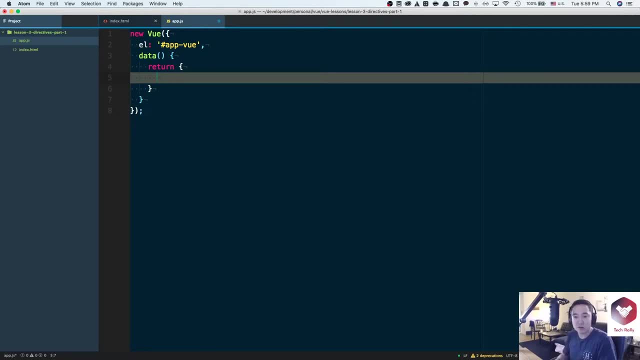 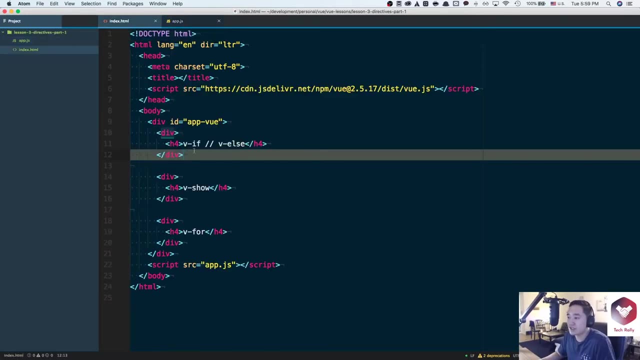 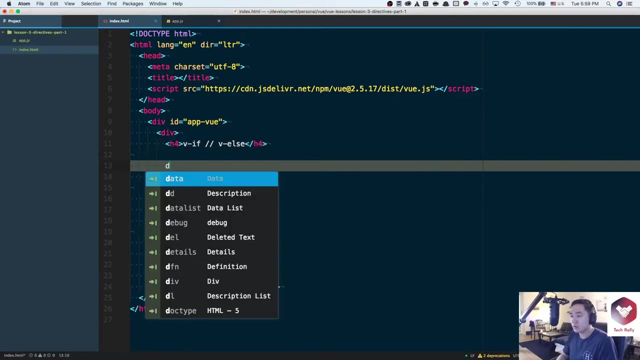 So for our purpose and example we'll use, I'll create a variable called if boolean and set it to true. Now I go back to the index dot HTML And basically this is where I will be kind of showing you how the VF directive works. So if I do div and then showing information via VF, 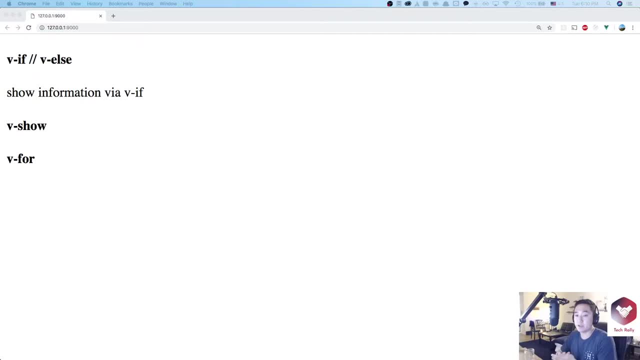 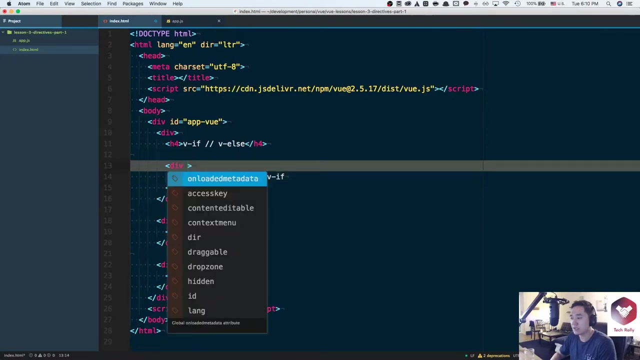 So if I run the server right now, what's being shown is plain old HTML. it just shows the text that says show information via VF. But what if we attach a directive specifically VF? I want to target this container that has the text show information via VF. So let's say VF. 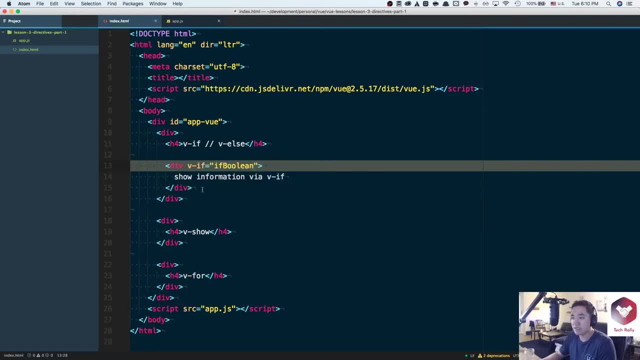 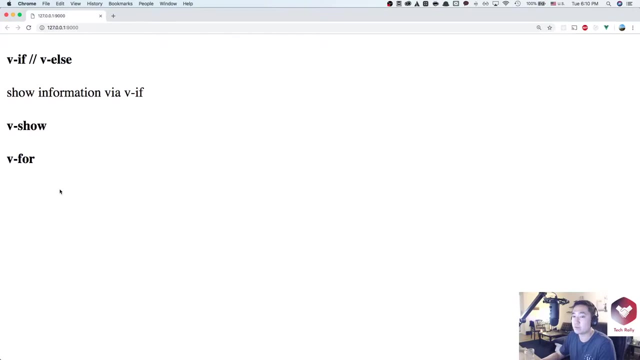 equals if boolean. What this is now doing is, if the if boolean variable is true, then show the content inside of it. And just to recap, in app dot j s if boolean is set to true. So when we look at the data, when we look at the rendered output, nothing has really changed. But if we go back to app dot, 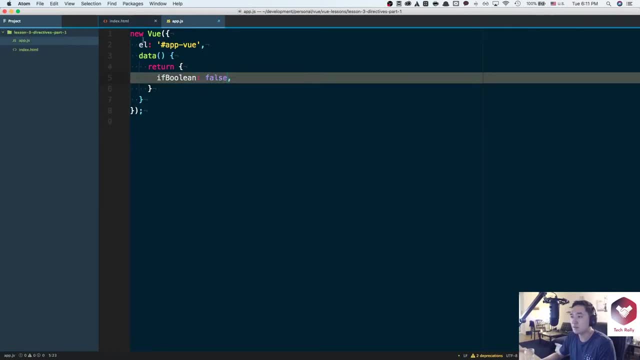 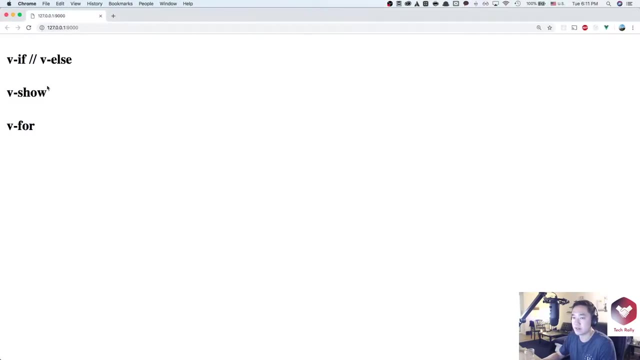 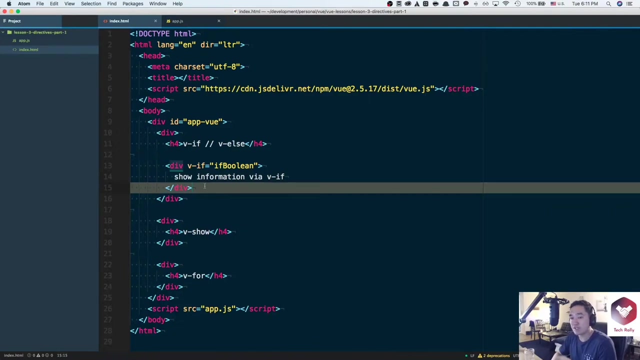 j s and set that if boolean value to false, it now says: if if boolean is false, then don't show this data, which is kind of like how it's being shown right here. we could take it even one step further and say: if you're false, and I want to show some other data, you could do another div. 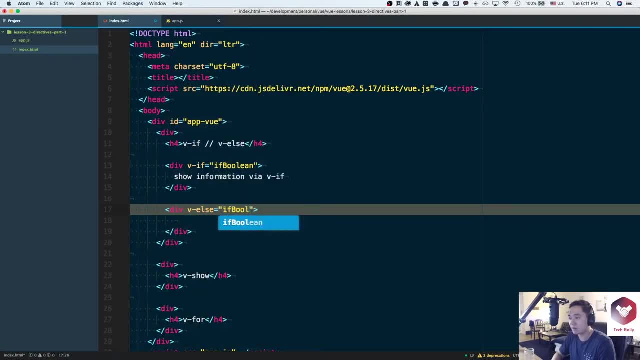 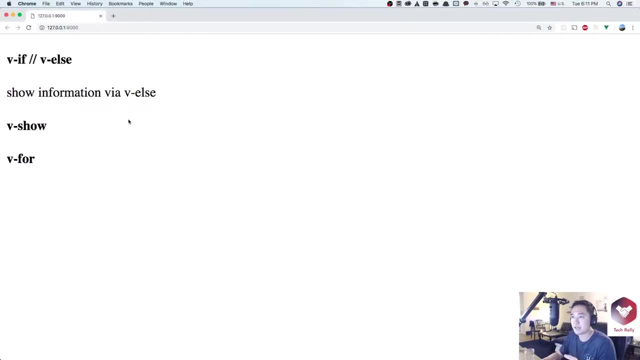 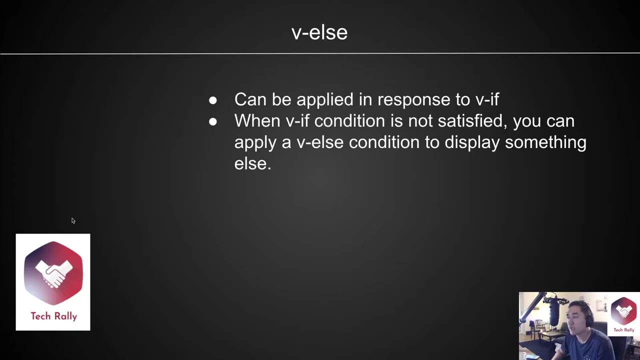 and attach a VLs to that same exact variable. So show information via the else. Now, if I look back at the rendered output, it's showing the data, since the original conditional fails To recap. velse can be applied in response to a vif. When a vif condition is not satisfied, you can apply. 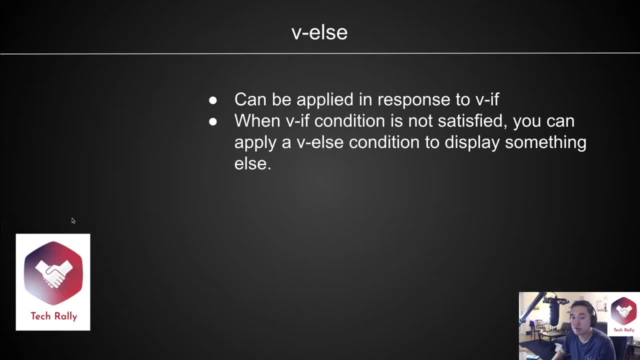 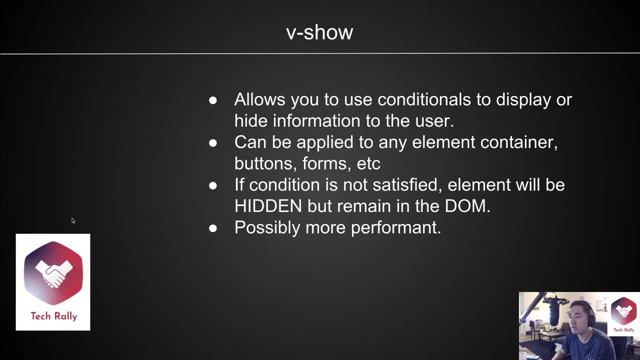 a velse condition to display something else. The next directive I want to go over is vshow. A vshow allows you to use conditionals to display or hide information to the user. If the condition is not satisfied, the element will be hidden but remain in the DOM. 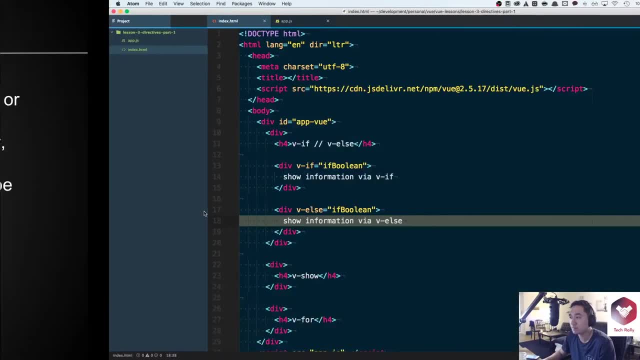 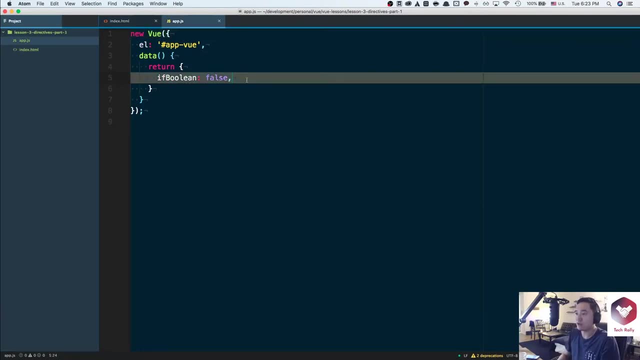 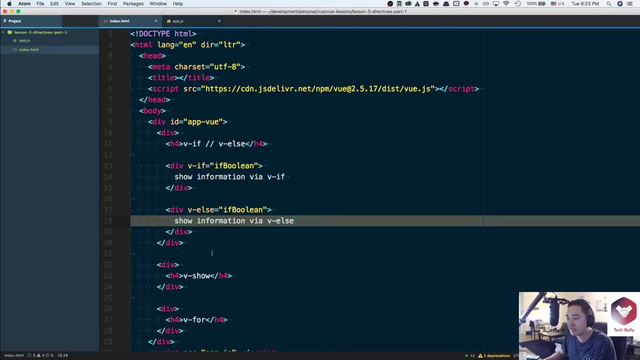 This can be possibly more performant. Let's look at an example. In the appjs we'll add another variable called ifshow, or we'll call it showBoolean, and we'll set it to true In the indexhtml. let's just do all of our vshow directives inside of. 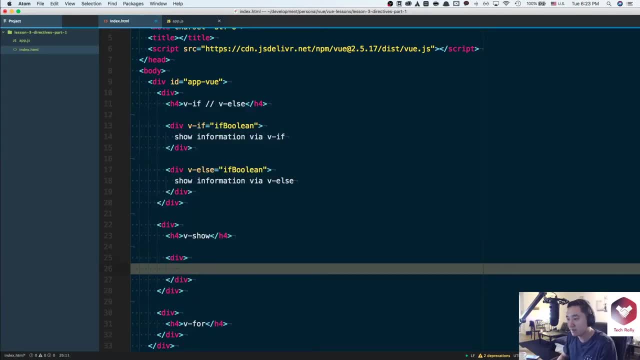 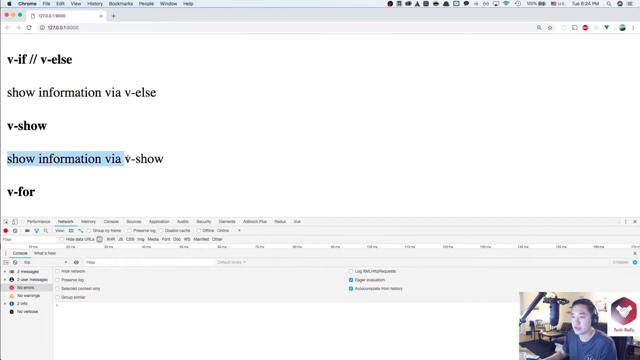 here. So let's create another div and then show information via vshow And then we'll attach a vshow to the showBoolean. So basically, if we go back here, then, yes, the show information via vshow will show up. 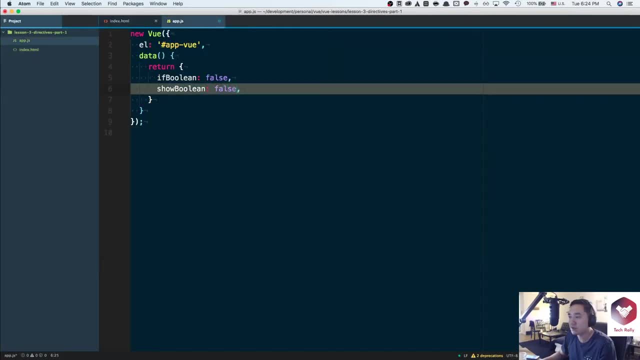 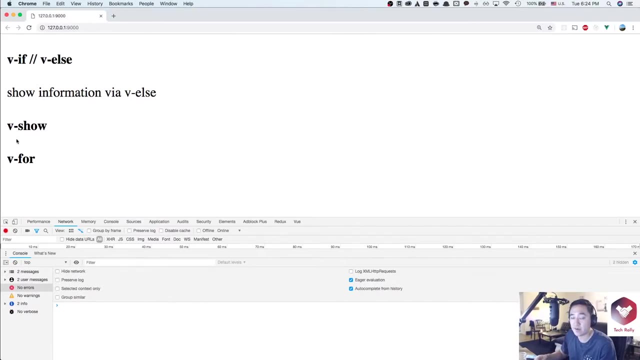 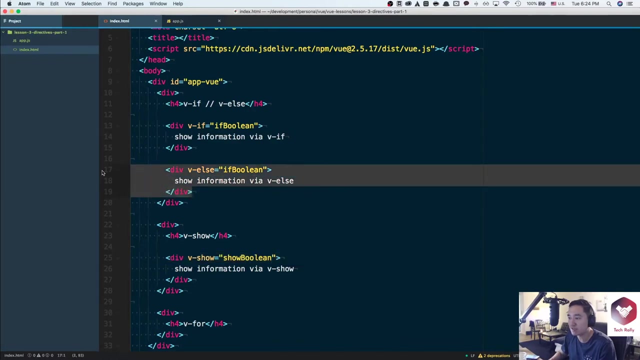 And then if we set the showBoolean to false, then no content will be shown. So what's the biggest difference between a vif and a vshow? Let's take a look. If I set the, if, if I remove the velse contents, 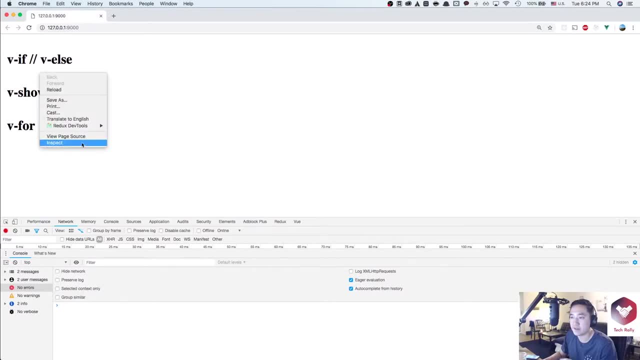 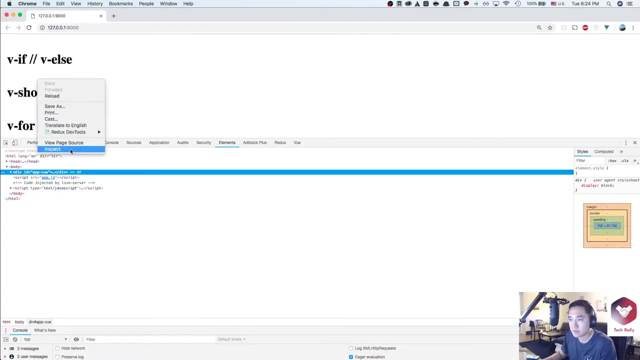 and then look and do and do an inspection on vif and vshow. Let's open this up a little bit Specifically. right here we have a div app view. we have the div. if You can see that the vshow is actually hiding the information from the user. 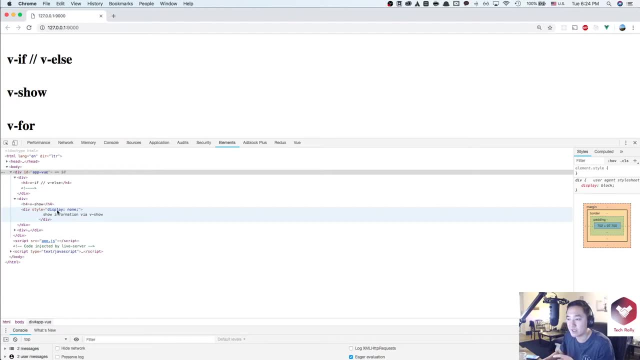 using CS or using inline styling called display, none, But, in contrary, the vif is actually removing it from the DOM itself. So, in in the case that you need to keep navigating back and forth and show or toggling back and forth certain data sets- and you know that you're 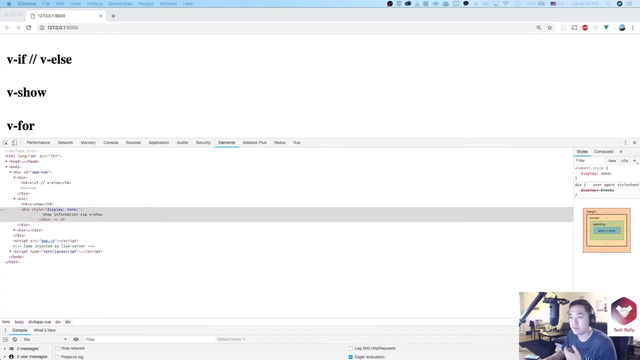 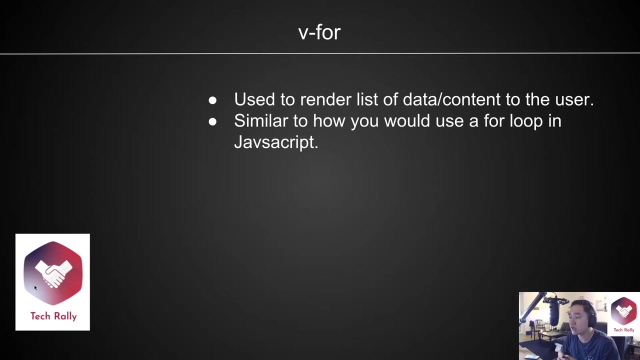 going to be doing often. it actually might be better to use a vshow instead of the if, because when you're adding and removing elements in the DOM, it could get very expensive. The next directive I want to go over is the v, for it's used to render a list of data or content. 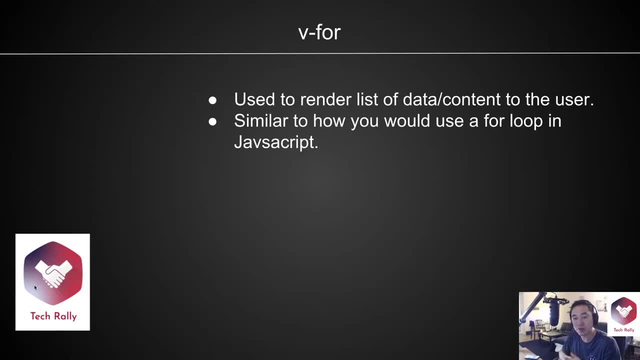 to the user and as a front-end developer, where you're required to probably make a lot of API endpoint requests and just return a list of data sets, this will be essential for displaying data to your user. in terms of usage, it's very similar to how you would use a for loop in JavaScript. let's take a look at the 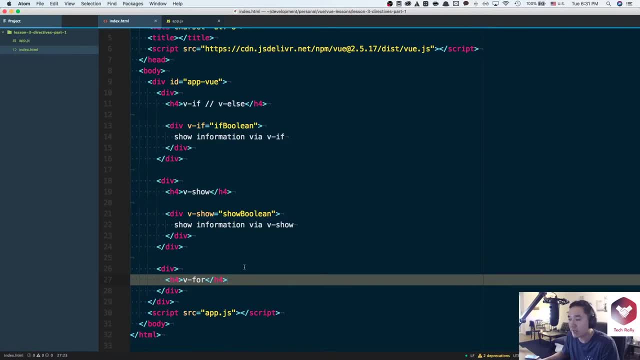 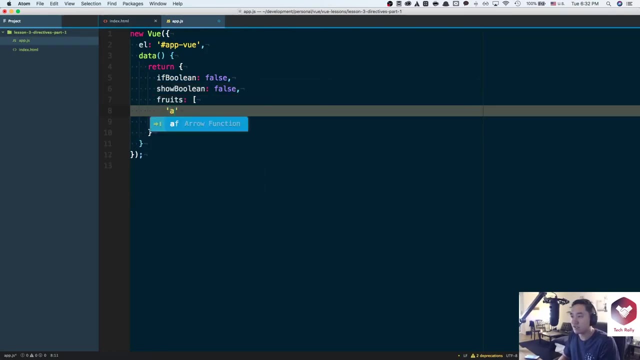 example. so here and we have the div with the h4, v4, but let's actually go into the appjs and create maybe like an array of items. so here I'm just gonna call it maybe something like fruits, and in the fruits there could be an apple pears. 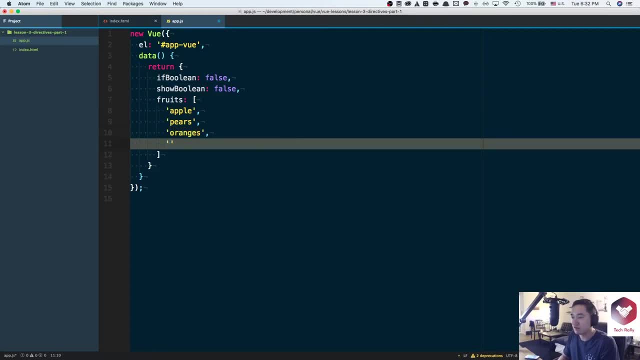 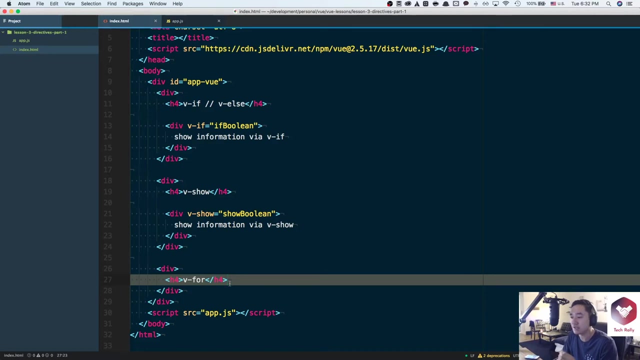 oranges. I think that should be fine, cool. so now this view instance has a data set called fruits and inside of this specific div I want to show a apple, pears and oranges as a list. so we'll create an unordered list and then technically what we really want to do- it feels regular, plain old HTML- would be. 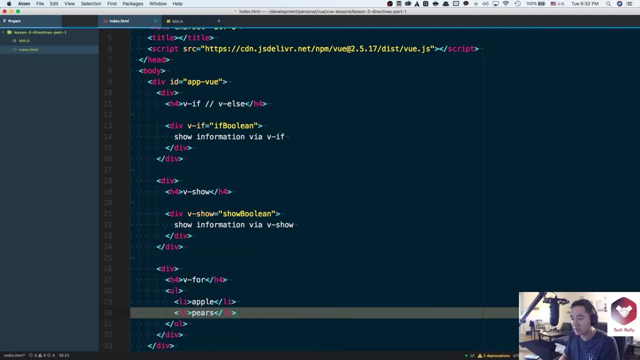 something like apple, pears, oranges. but obviously we can't do this when we're making endpoint requests and getting data from like a server, because this is just strict HTML. so to account for this view provides us with the view with the v4 directive, so what instead we could do is now attach a v4 and add some content. 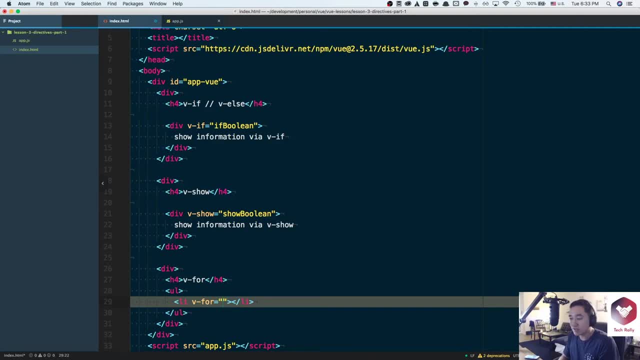 inside of these quotations. so in our case we're gonna say: v4 equals fruit in fruits, and fruits is actually coming from the appjs that we've defined in the data set, and fruit it's just a random variable name that I decided to do, but you could call it whatever you want. you could call it my fruits fruitsjavascriptjparatypeline О Moto V4.jangles.